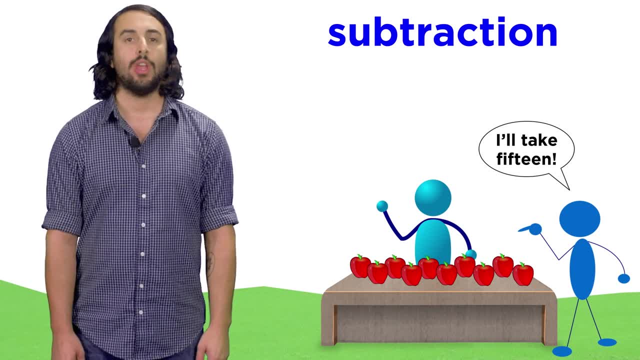 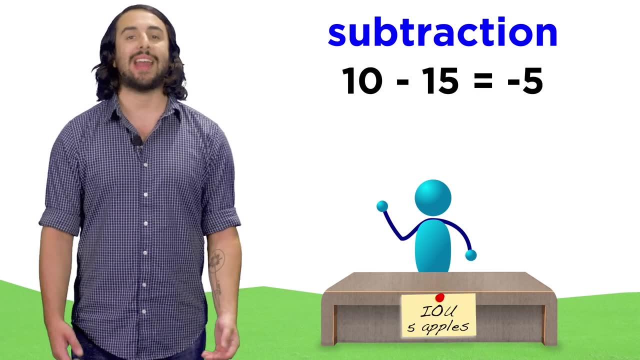 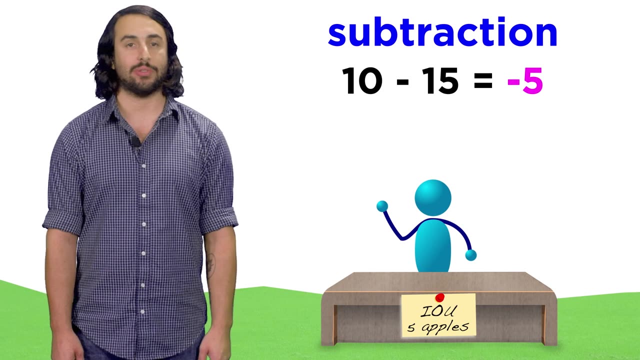 Let's say someone wants fifteen apples. You could promise them fifteen apples, saying you'll get five more tomorrow. So in a sense you could say that after the transaction you have negative five apples, which is five fewer apples than no apples. 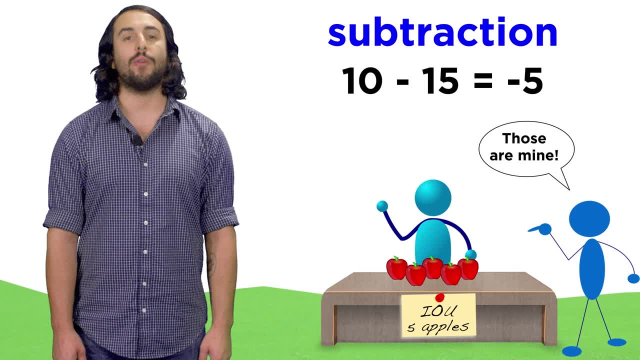 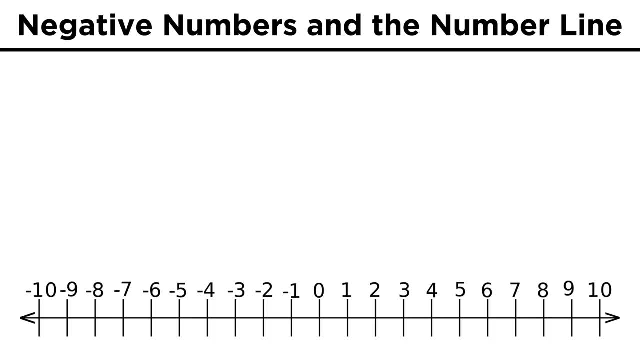 This is because once you get more, you immediately owe five of them, so it's like you will need five apples just to get to zero apples. To make sense of this, let's look at a number line. Until now, we've been looking at the positive side. 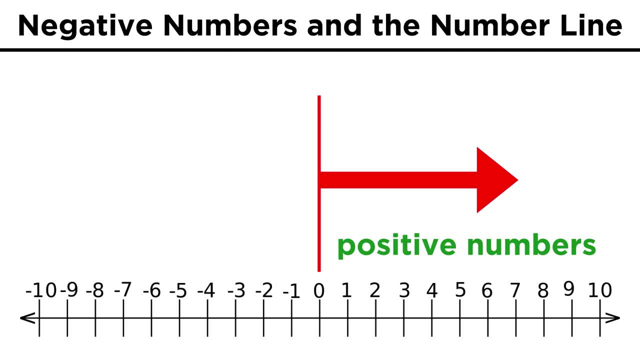 The negative side, which continues climbing all the way to infinity. But on the other side of zero, if we continue subtracting, we start with negative one and we can go all the way to negative infinity. This helps us understand the magnitude of negative numbers, because numbers to the right. 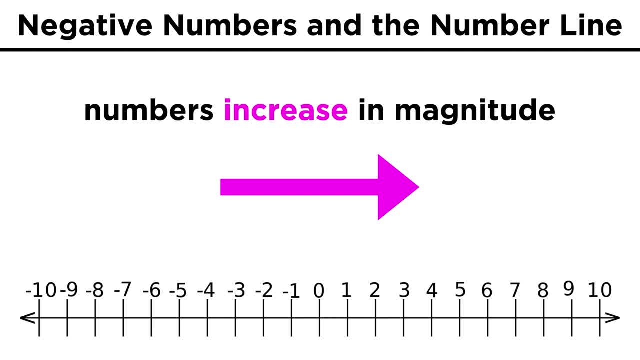 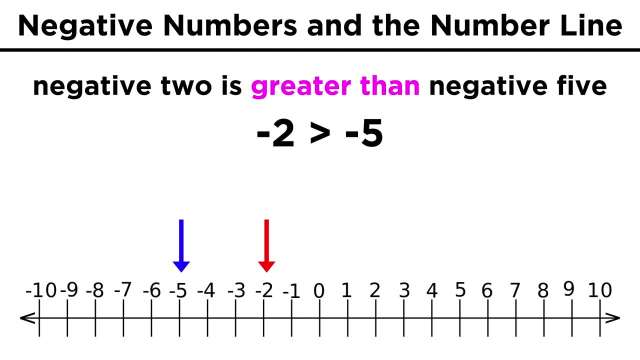 on the number line are always greater than numbers to the left. This means that negative two is greater than negative five, which can be counter-intuitive, Because five is greater than two. But if you picture the number line in your head, it will always make sense. 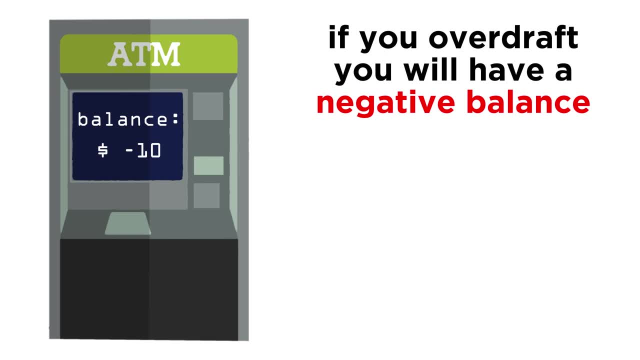 Think of your bank account. If you overdraft, your balance will be in the negative, and if you owe the bank ten dollars, you have more money than if you owe twenty dollars, because you will need less money to get back to zero. 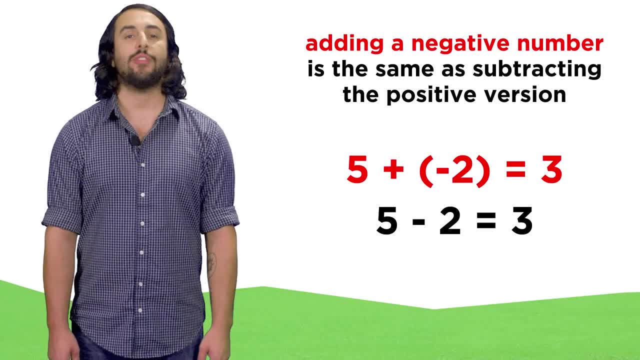 Now let's try some operations with negative numbers. If we are doing addition, adding a negative number is the same as adding a negative number. Adding a negative number is the same as adding a negative number. Adding a negative number is the same as adding a negative number. 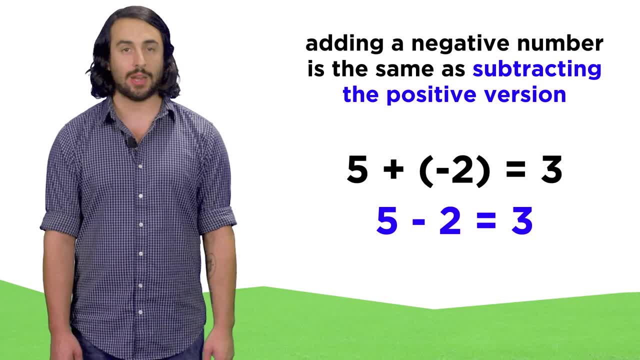 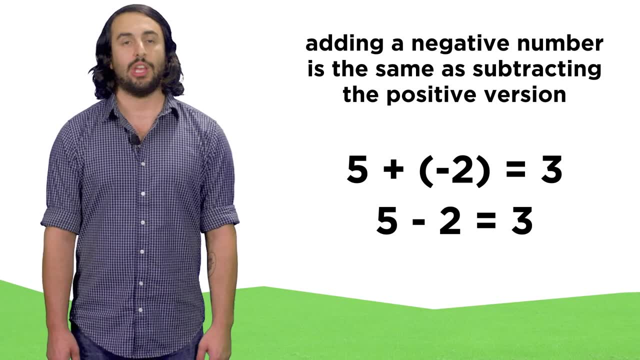 Adding a negative number is the same as subtracting the positive version of that number. Five plus negative two is the same as five minus two, which gives us three. If we are doing subtraction, subtracting a negative number is the same as adding the. 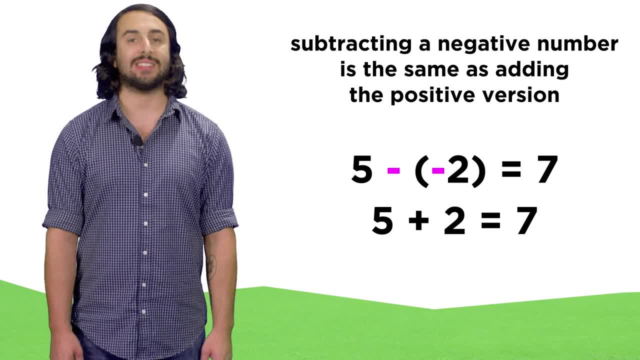 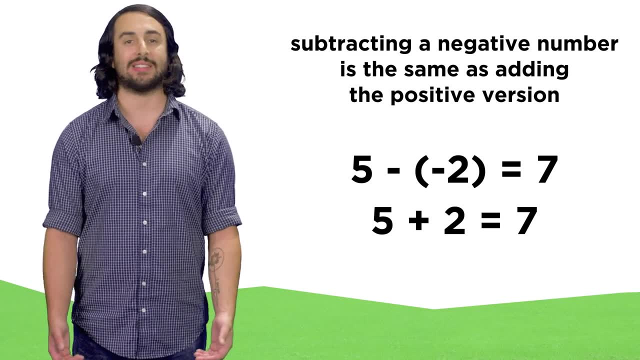 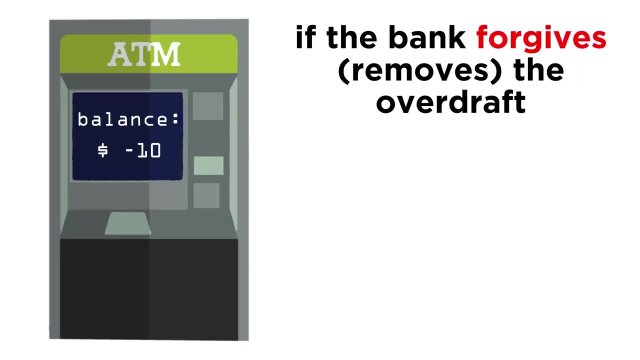 positive version of that number because the minus signs cancel each other out. This cancellation isn't magic. it actually makes perfect sense because taking away a negative amount is the same as subtracting a negative number. If your bank account is overdrawn by ten dollars and the bank were to forgive or subtract that, 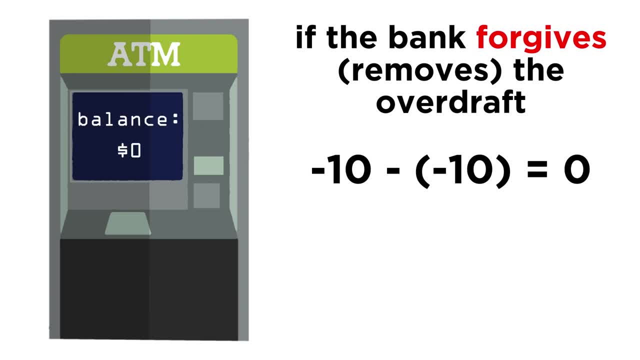 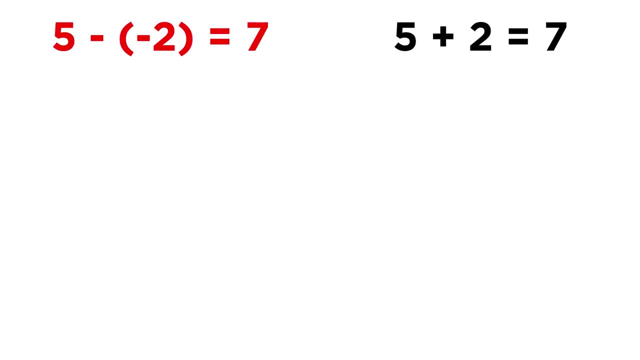 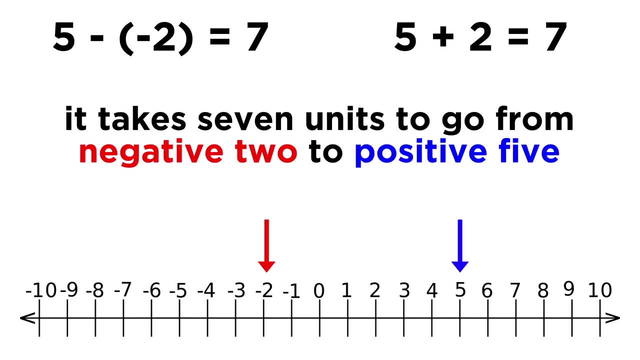 overdraft, you'd suddenly be at zero, which is ten more than negative ten. so it's like the bank gave you ten dollars. So five minus negative two is the same as five plus two, which gives us seven. We can even verify this on the number line, as there are indeed seven units between negative 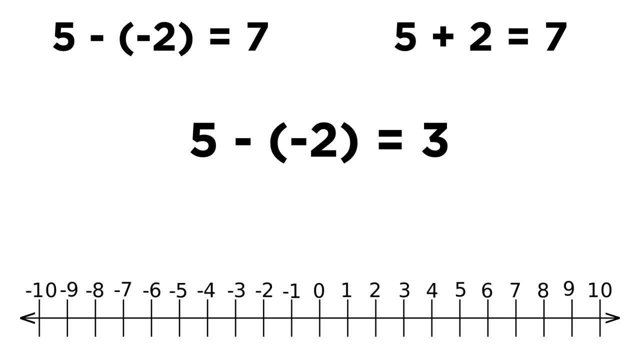 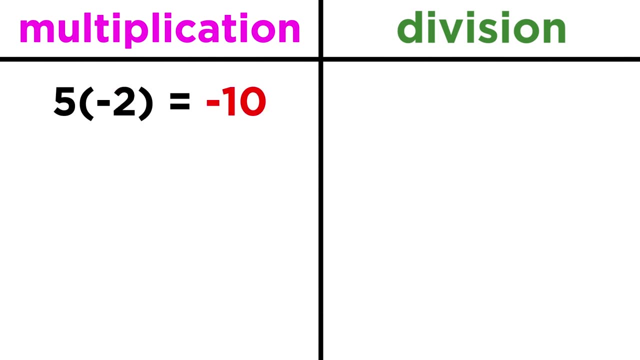 two and five. Incorrectly subtracting negative numbers is a very common source of error for math students, so make sure you don't make these kinds of mistakes With multiplication and division. if one of the numbers is negative, the answer will be negative. 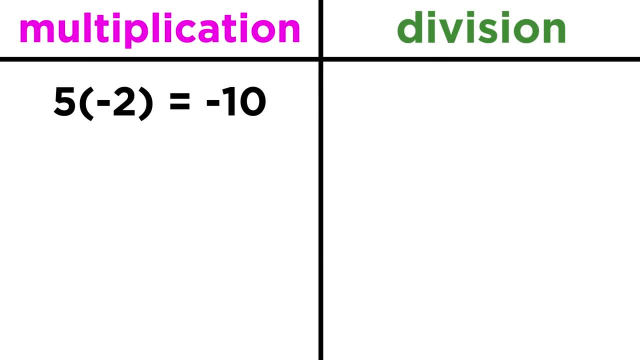 Five times negative two is negative ten, which makes sense, since adding negative two five times will give us negative ten. Similarly, fifteen over negative three is negative ten. However, if both numbers are negative, again the minus signs cancel each other out and 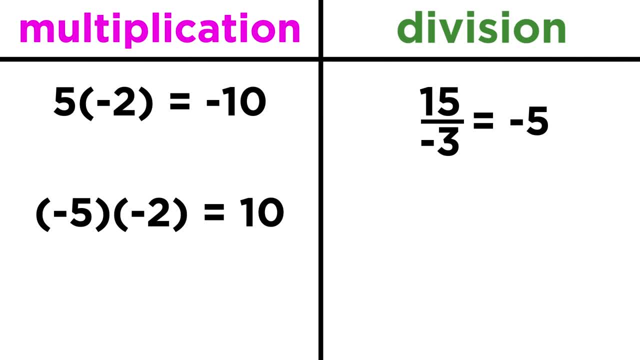 the result will be positive: Negative five times negative. two is positive ten. Negative fifteen divided by negative three is positive five. This makes sense if we think of each number as negative one times the positive version of the number. Negative one times fifteen. divided by negative one times three is correct. 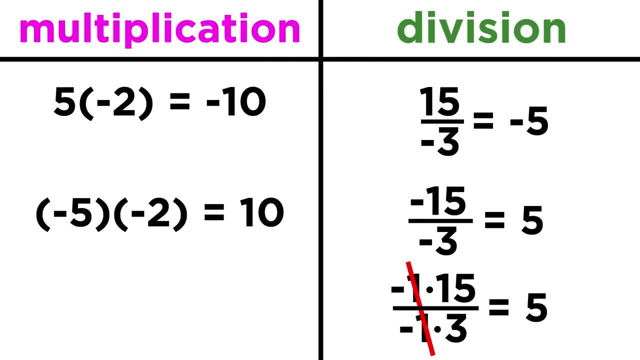 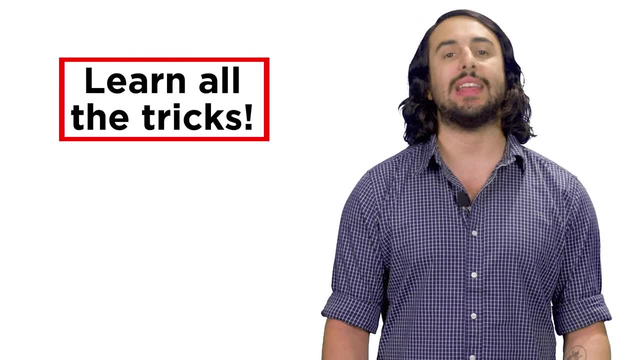 Negative one times fifteen divided by negative one times three is correct. Negative one times fifteen divided by negative one times three is clearly positive five, because the negative ones cancel out, since anything over itself is one. Little tricks like this make it easier to remember all kinds of arithmetic identities. 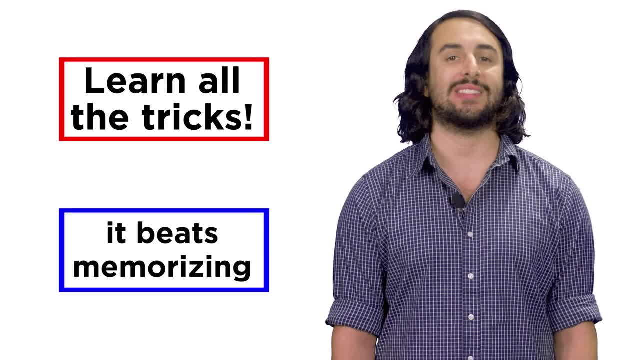 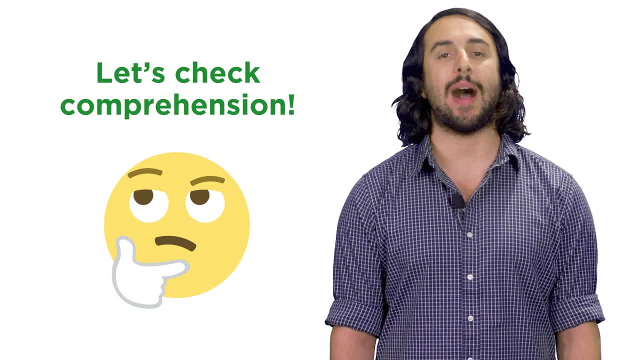 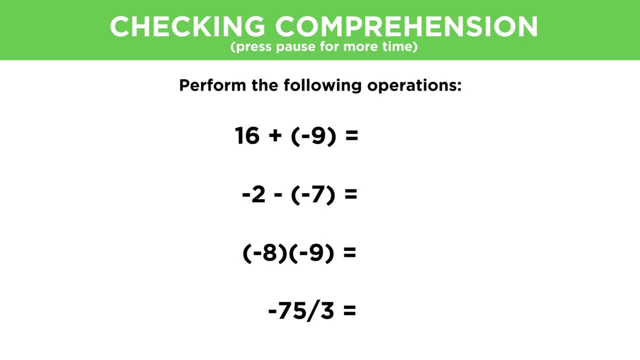 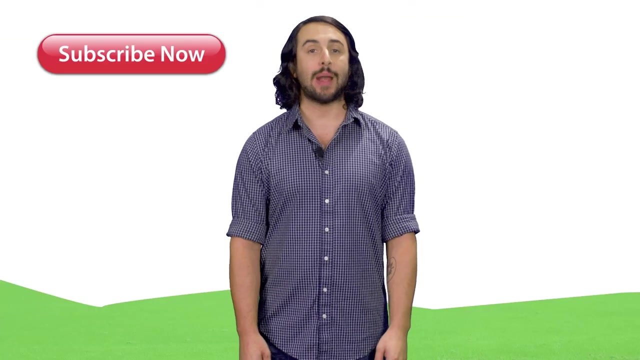 and help us go beyond simple memorization, which by itself doesn't always lead to a deep appreciation of mathematics. Now that we know how to perform operations with negative numbers, let's check comprehension. Thanks for watching, guys. Subscribe to my channel for more. 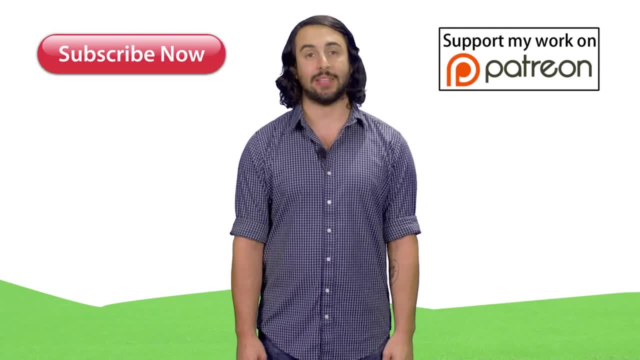 I'll see you in the next video. Bye.